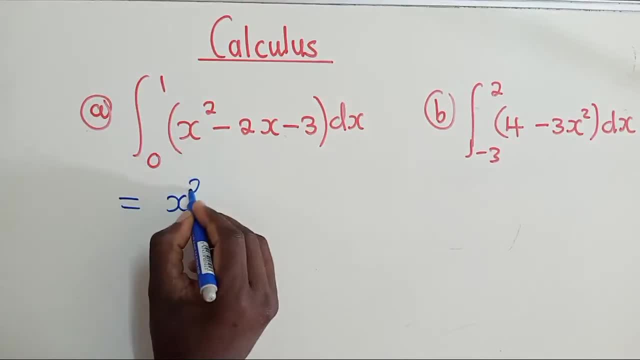 You just say equal to X the power which is here at the one. So We have a two here, So it's a two plus a one, and then divide by the new power which is right here. So whatever you have here, divide like that. then you say equal to X, right here. 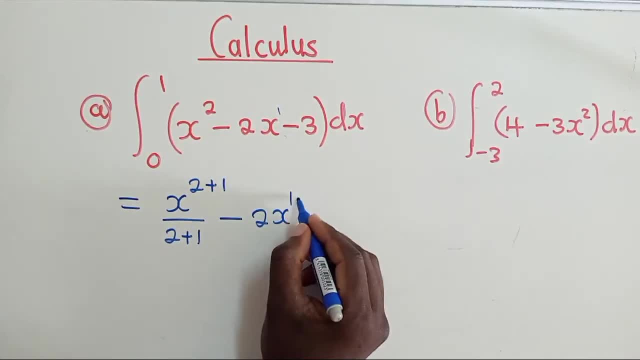 What part do we have here? There's a power one, of course, here. So it's a power one. You add the one. You always add the one. The rule is that you add the one. Okay, John. Thank you so much, John. 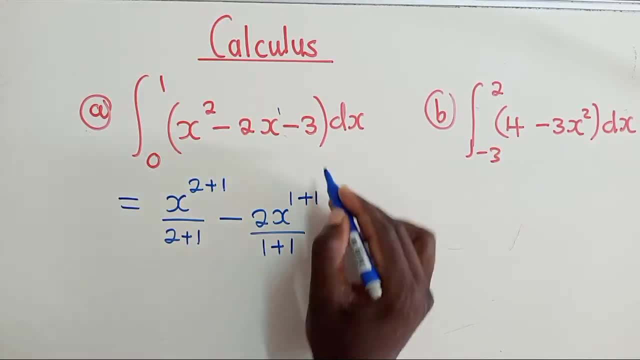 The next thing: you divide, just like that. Then, here you have a three. So what do you do? Do we see any letter here? No, So what are we going to do? Just get this same three and the letter that you are respecting. 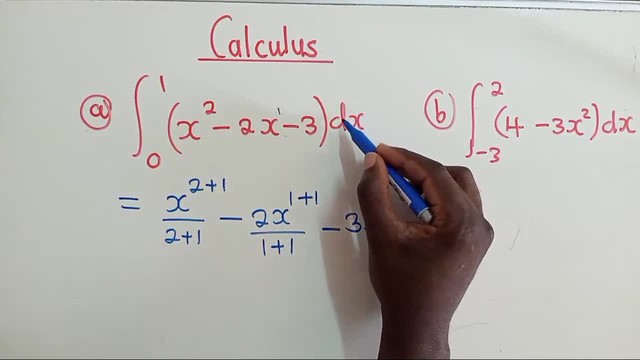 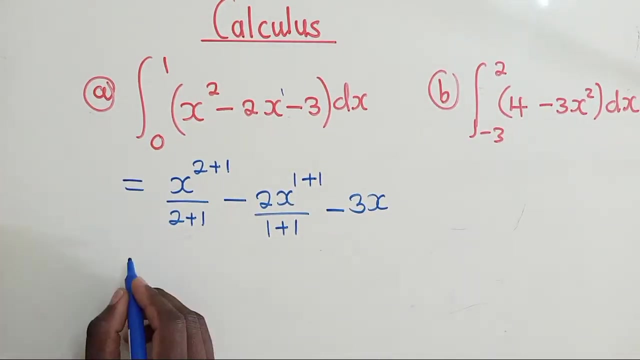 In this case it's X, So we are respecting X. where there is DX, Just get the letter which is here and put it there, And this is what we have. So the next thing here will be to simplify. So we simplify. 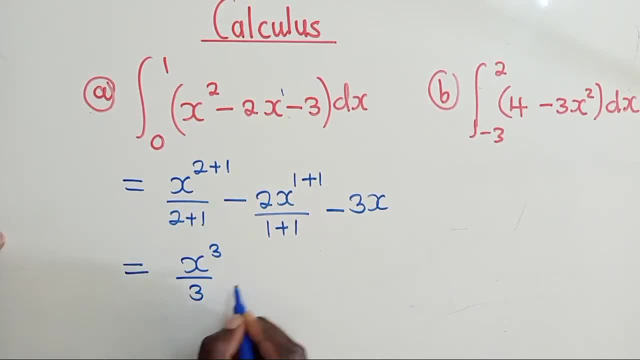 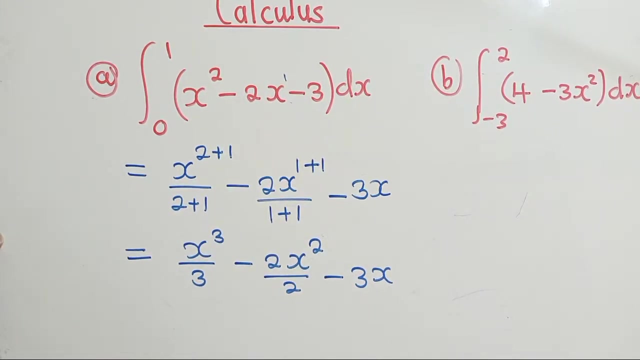 We shall have X power: three over a three minus two. X power: a two. One plus one is a two over a two here, minus a three X. Okay, Jimmy, Thank you so much, Jimmy. I see you Next thing. here is the same stuff we have. 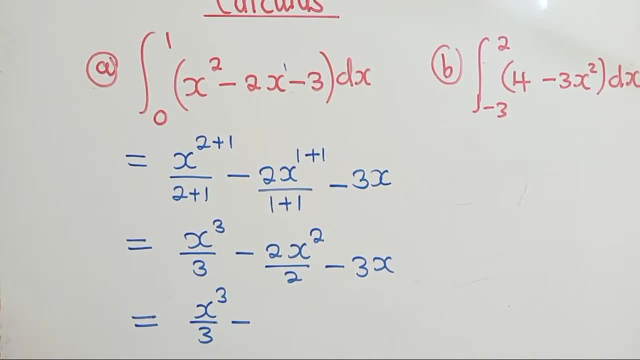 And here, If you You are able to see, nicely, there is a two here and this two will cancel. We shall remain with X power two minus three X here, Just like that. I guess it's okay up to here. It's okay up to here. 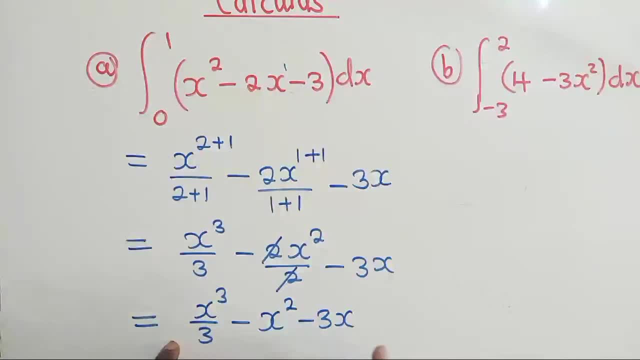 So now, after reaching this point, what do we do next? Apply the brackets like this: On top here you put a one Okay, Because the up here, Here, Here, Okay. So that's the thing. Is it okay? up to here. 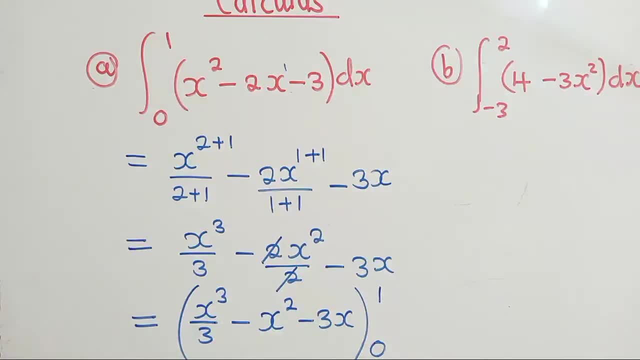 Is it okay up to here? Kindly confirm if it's okay. Abubaka, Is it? Ah, sorry, Abubaka. Yeah, that's Abubaka. Three under this, Like that. Okay. Okay, I guess you're able to. 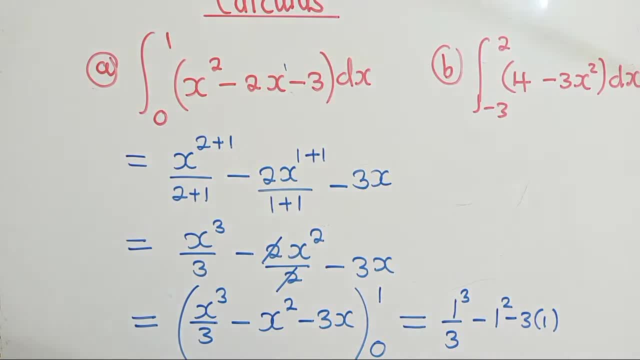 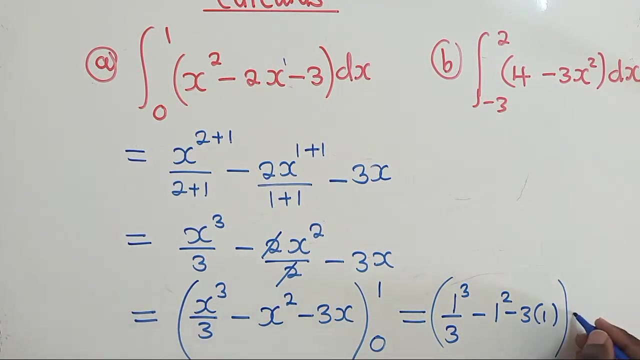 Okay, I guess you're able to follow what is happening. Okay, So here you even apply the brackets like that. Okay, You put the brackets like they were put here And then you say minus a zero. Okay, So when you do that, you just simply simplify here. 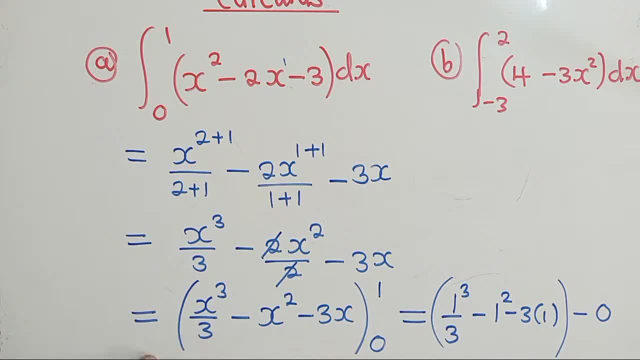 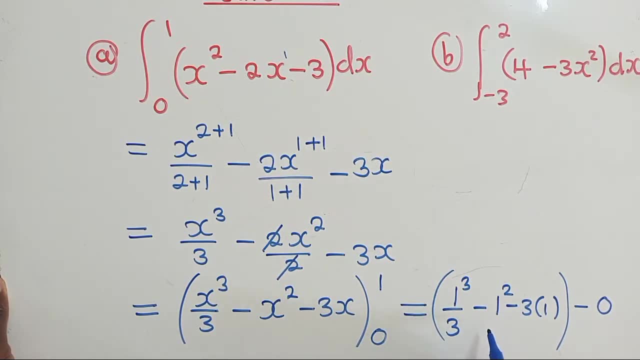 You simplify right here, Okay. So when you simplify here, what are you going to get? You're going to get from here, Okay, We're at this stage. So when you simplify from this stage, what is it that we're going to get? 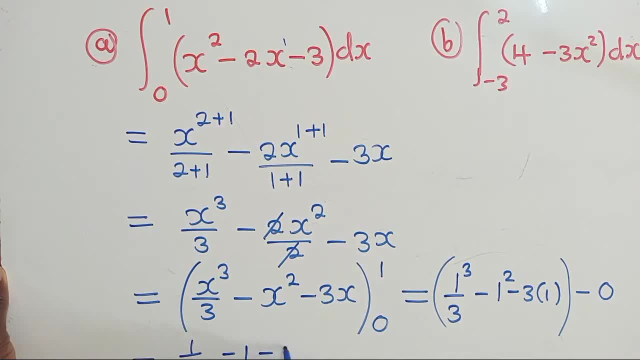 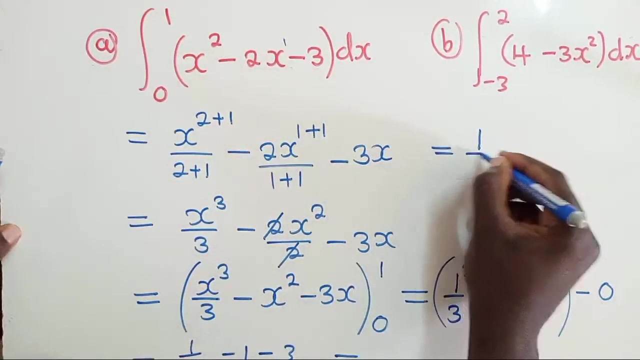 We're going to get a one over three minus one minus a three. This is a zero there, which is equal to. So let me copy so that we see nicely from this stage. So I'll put it here from this stage: One over three minus a one minus a three. 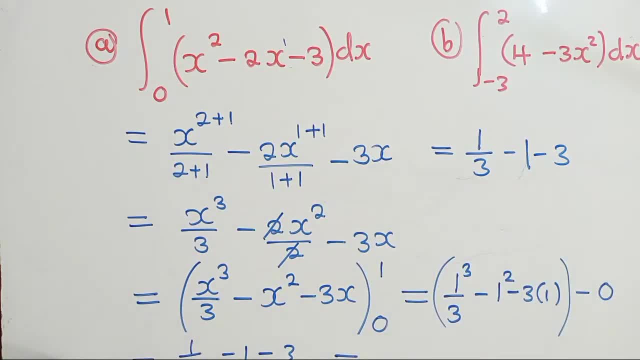 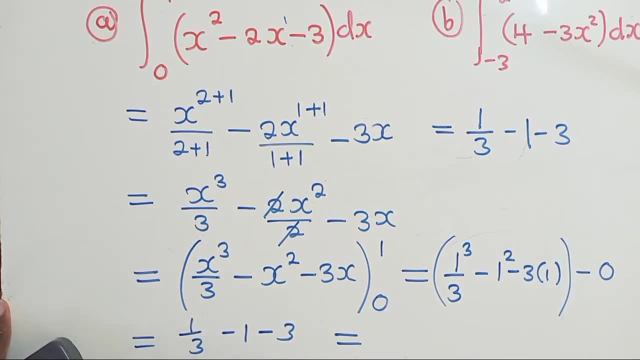 So I've just copied this and put it here So that we see the way it will look like. Okay, I guess you are following. So now, from this stage, because we're at this stage, now after substituting. we're at this stage. 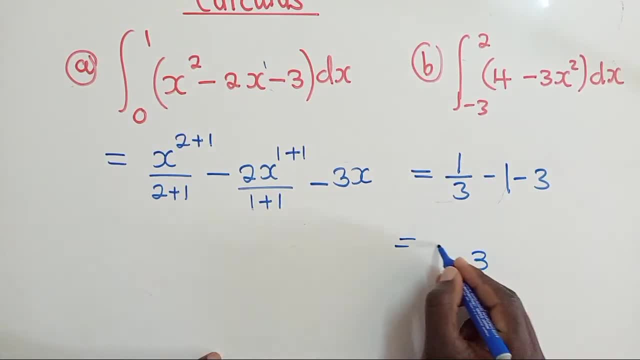 So, from this stage, we find the lowest common denominator, which is a three, three, two, three. one there, You should have a one here. It would be a negative three here, Negative nine, Because there's a one here. 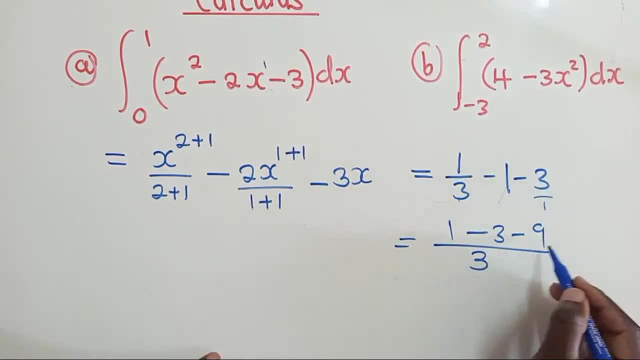 One into three is three. Three times negative Three is negative, Negative nine, And when you simplify here, you should get negative eleven over three as our answer. That's our answer. I guess you understand up to here. So now we go to question B. 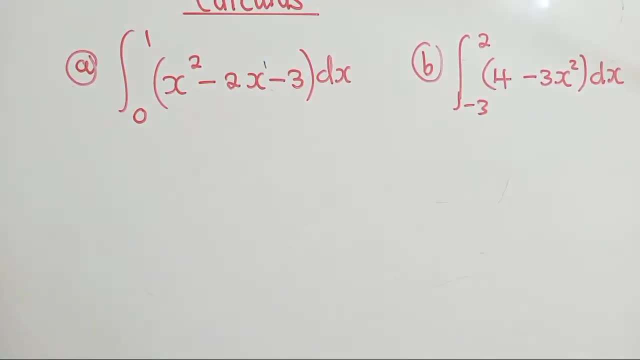 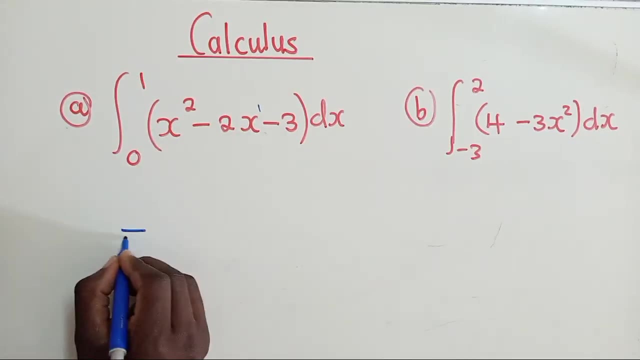 If it's clear, we go to question B. So the same concept, the same idea, The same idea for question B. So you should say equal to for this, This one, You should say equal to that stuff that we have here. 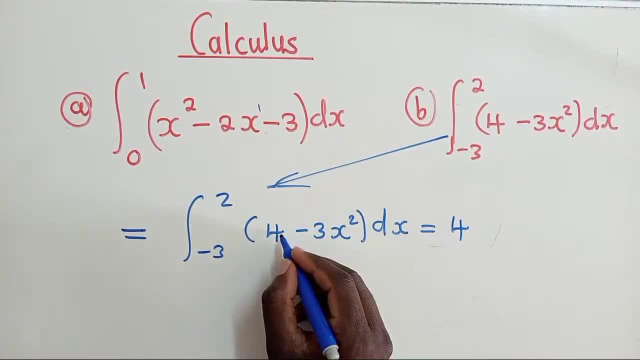 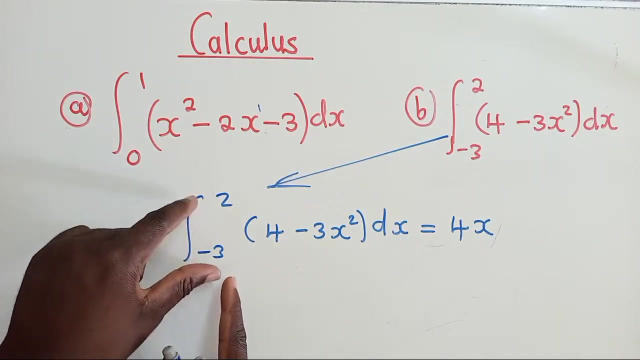 Do the same thing when you've got a constant here. So this is what we have. Okay, What is Howard saying? Why? subtraction instead of addition? You don't add. That's Howard. You don't add When this the difference? we find the difference between the upper limit and the lower limit. 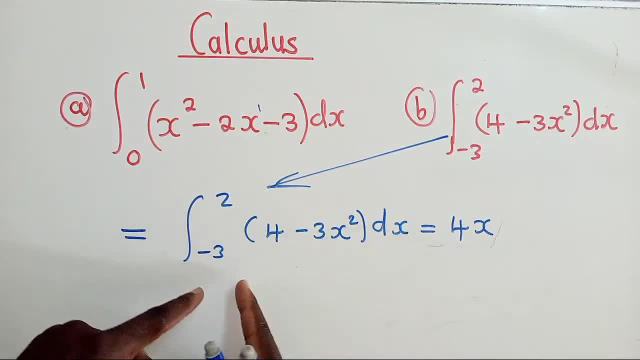 So when you substitute, for example, this, you plug it in, You come and say minus, You substitute the other one. So I'll explain on this one. So keep on following so that you understand. So we should have a three. 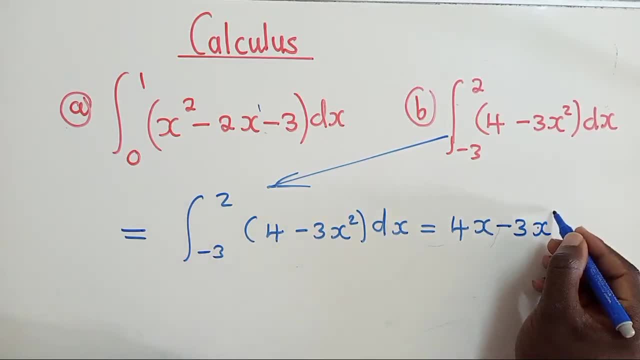 Negative: three there, X power. two plus one there over two plus one, Okay, Okay. So this is what we have here Now from this stage. From this stage, we should get a four, X minus three, X power, three over a three. 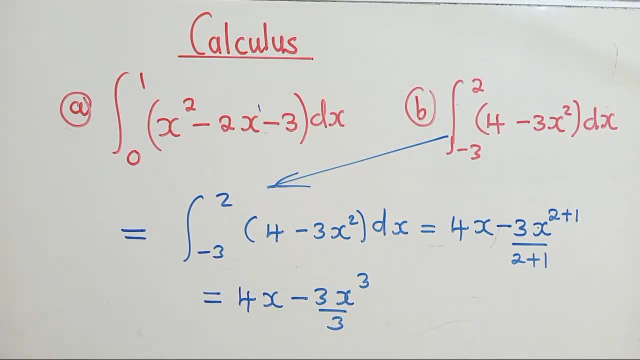 I guess you're following such that these three and the three here will cancel, So we shall remain with Four X Minus three X power three over a three Minus three X power three over a three Minus three X power three over a three. 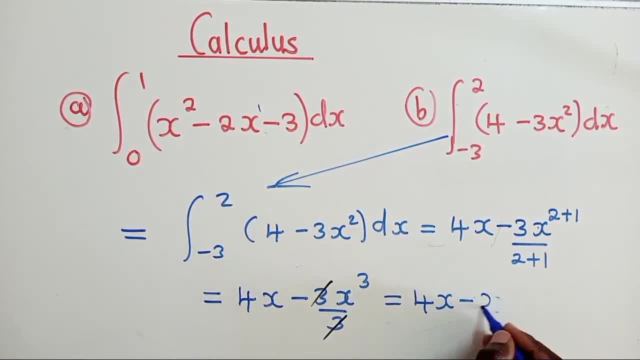 Four X minus minus X, power three. So this is what we have. We now plug the limits: Upper limit is a, two, Lower limit negative three. Remember, we are on question B. So that's the thing We are at this stage, where we are expected to substitute. 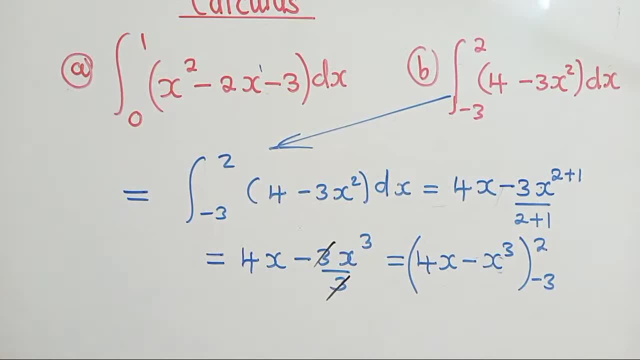 The next thing here will be to just say: for the upper limit is a two there, Minus A two, power three. You see, this is what I was talking about, the limit. So once you substitute this and this here, you say minus. 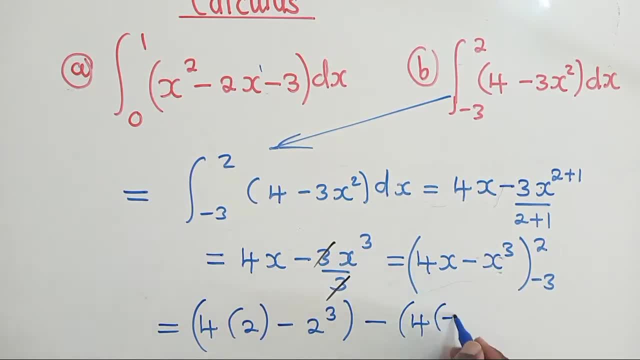 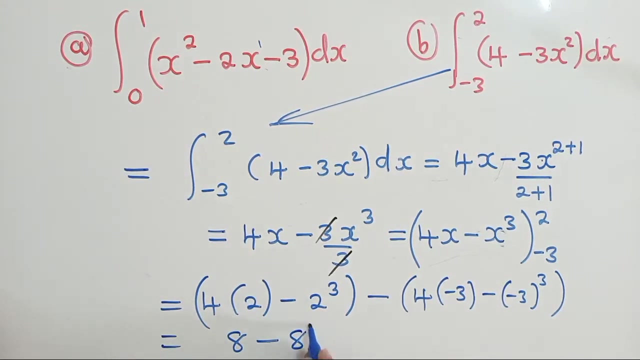 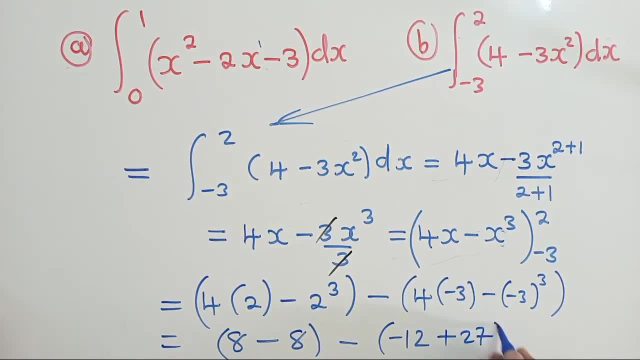 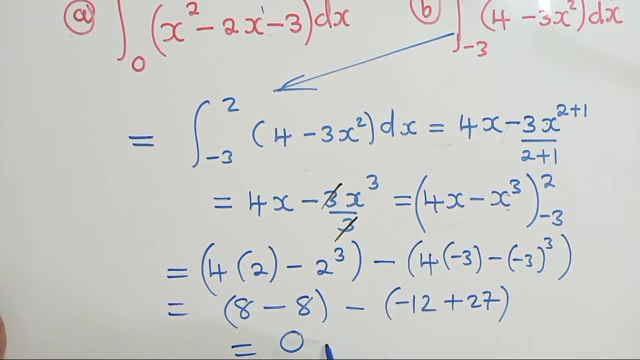 Minus here, Minus here. Here we're getting a positive 27. Okay, So this side will just be a zero. It will be a zero Minus here, It will be a 15. When you work out what is inside the brackets: